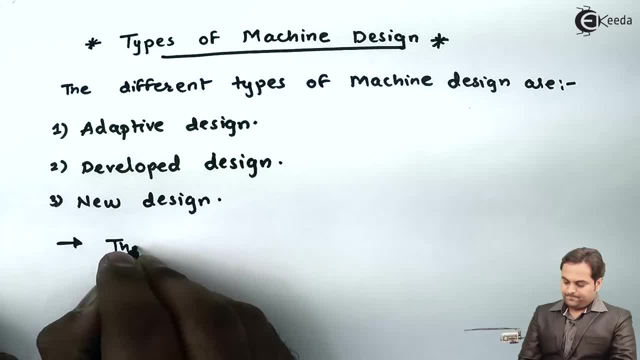 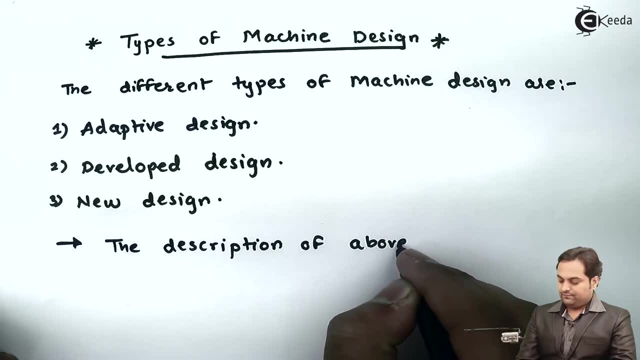 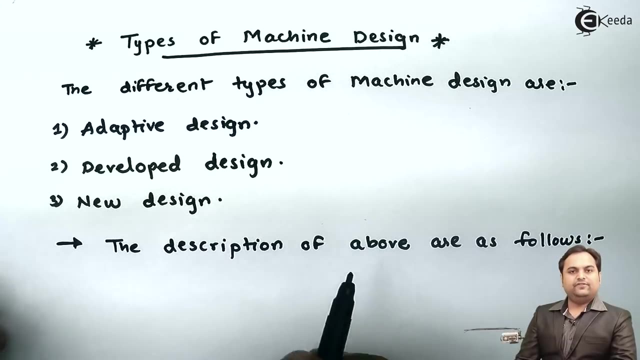 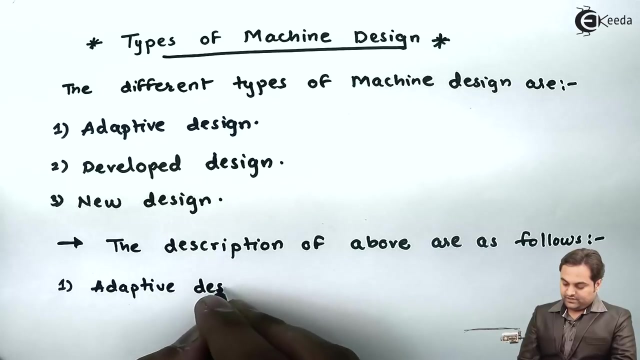 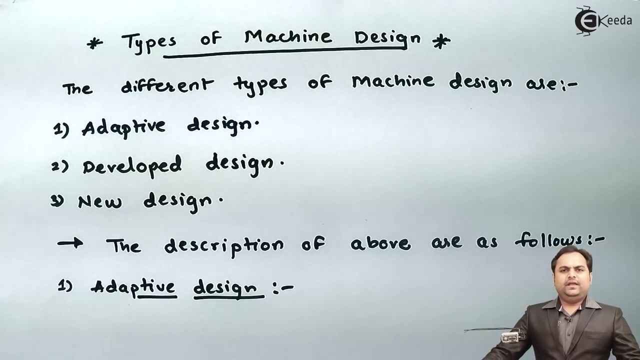 In detail, the description of above are as follows. I'll first start with adaptive design. Adaptive design Now see adaptive design. adaptive design is basically a small modification or minor change in the existing design. It means in case of adaptive here, the component or product. 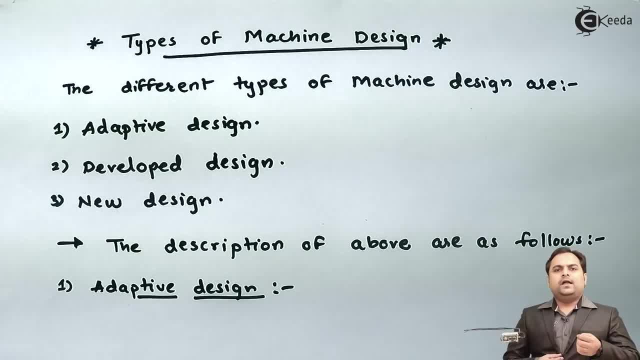 is already there, it is existing, And when we make minor changes in that, then we term it as adaptive design. In simple terms, if we can say adaptive design is not a new design or we are not designing any product from scratch, 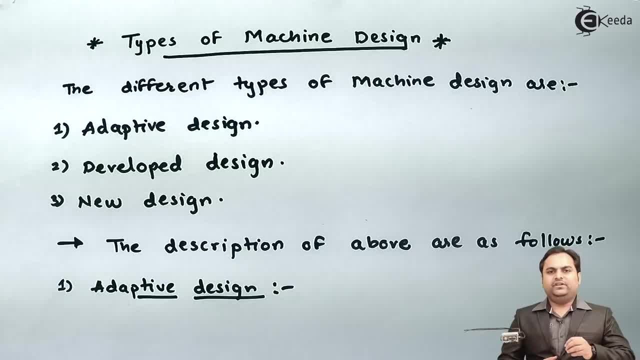 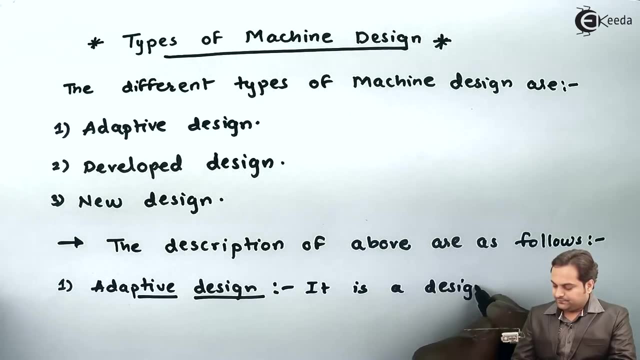 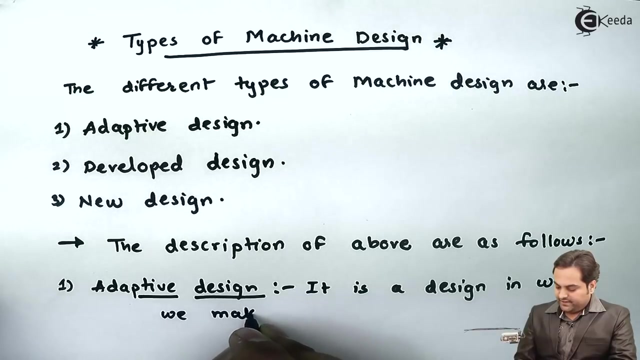 Here. some product is already there, but we have to just change it or provide some minor modifications. So here I'll write the definition that it is a design in which we make minor modifications. So we are making a new design and we are not designing any product from scratch. 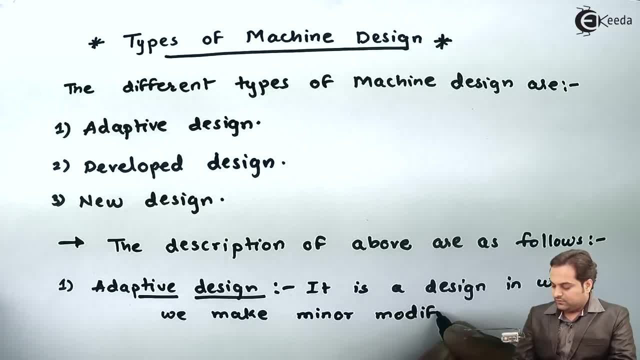 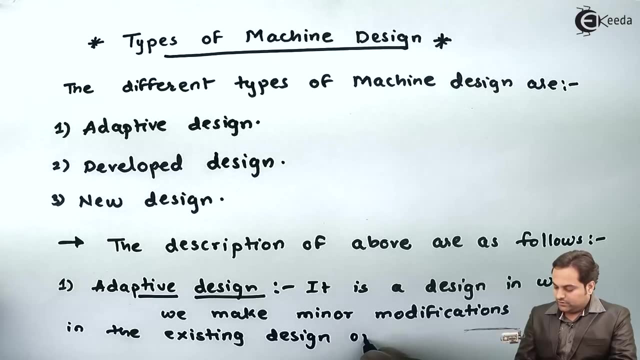 minor modifications in the existing design or product. so if we change slightly some design feature, like for example, if some product is there, if we are just changing its color, then it is called as adaptive design. or if we are adding some component, we are or we are removing some component, then also it. 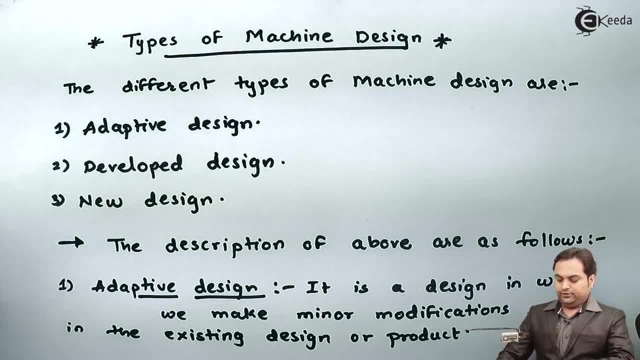 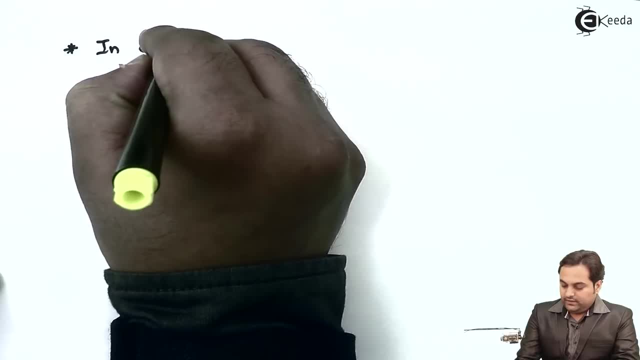 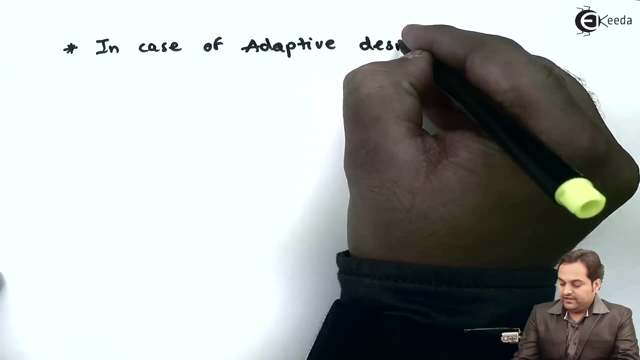 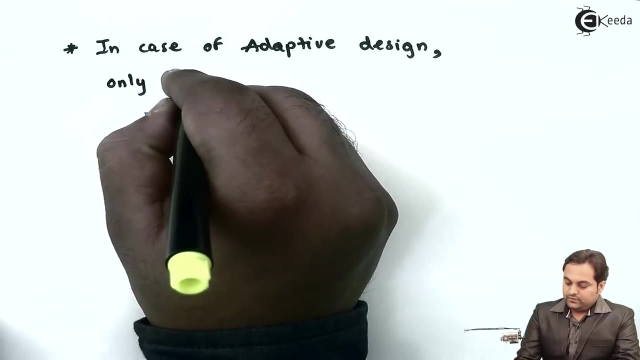 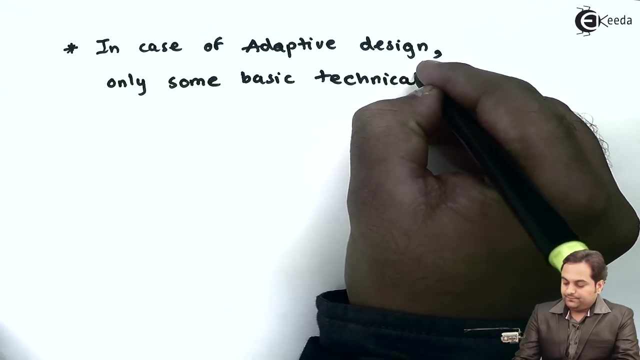 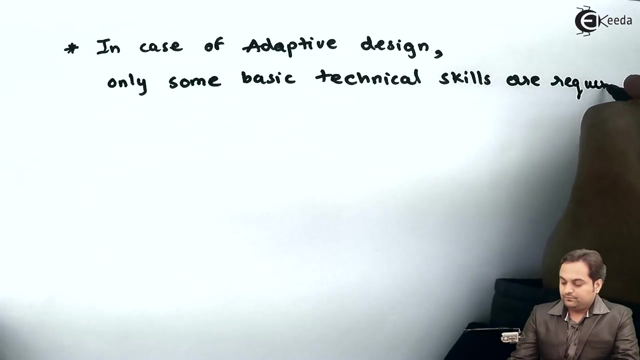 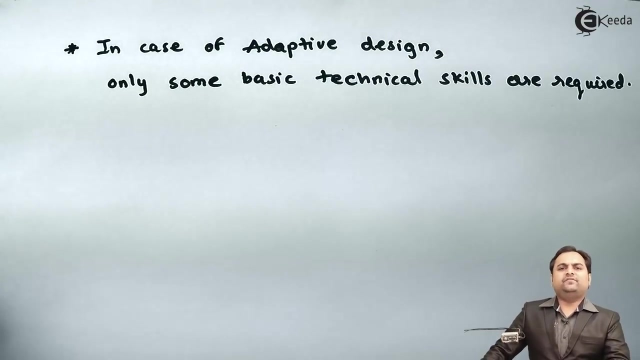 would be called as adaptive design. the next important point in adaptive design is- I'll write it here- that in case of adaptive design only some basic technical skills are required. so if a person he is an adaptive designer, then he should just have some basic technical skills to make any. 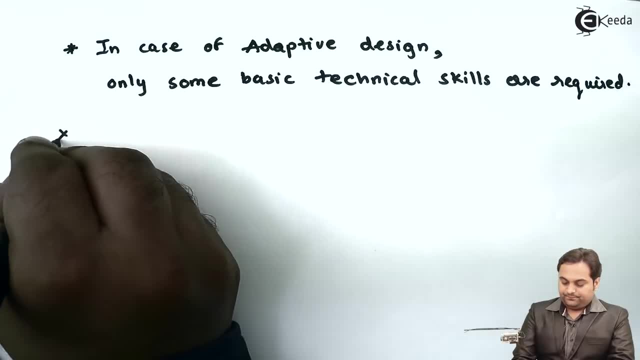 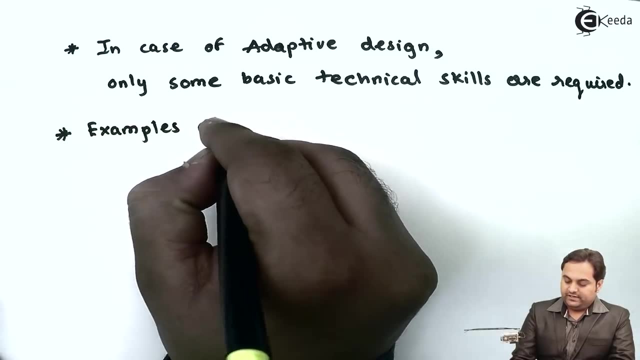 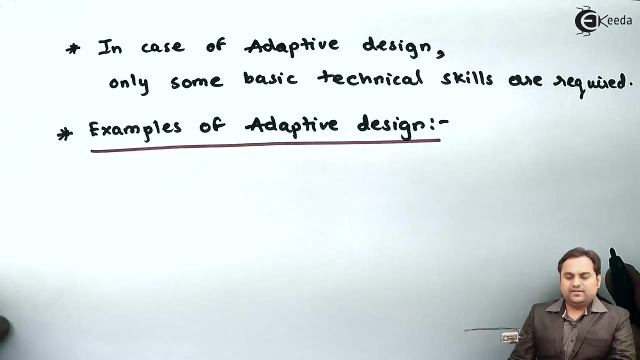 change in the design. here I can give the examples of adaptive design. the best example which I can give here it is of diesel engine. now, as we know, diesel engine is already existing, it is in use. make any small modification in a diesel engine, then it would be termed as adaptive design. 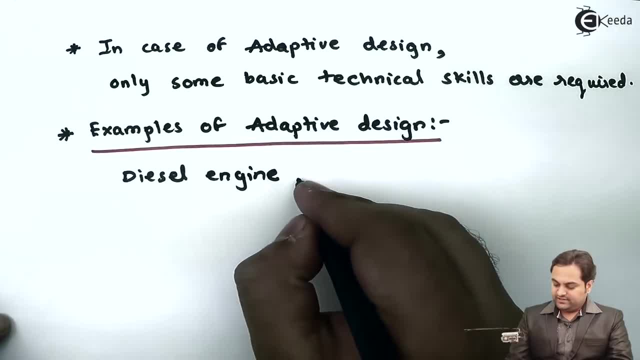 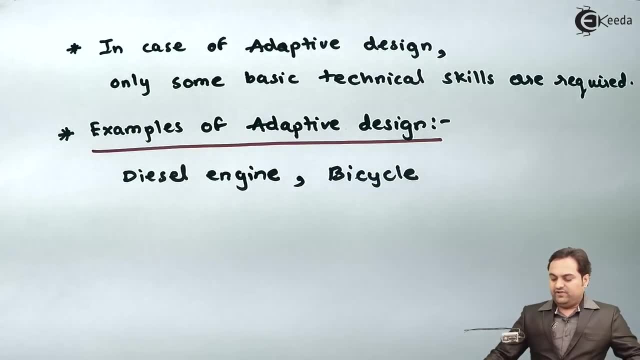 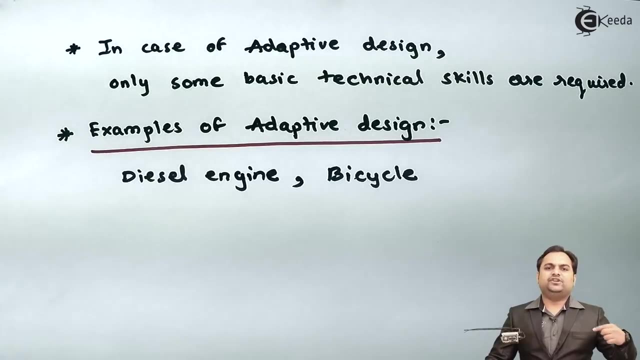 So diesel engine comes under the category of adaptive. Next, I can give the example of bicycle: See bicycle example. why I have given here? because previously we were having a bicycle which was driven by pedal and there was chain which was transferring the motion. Now, if we can see, there are even bicycles which are gear operated. 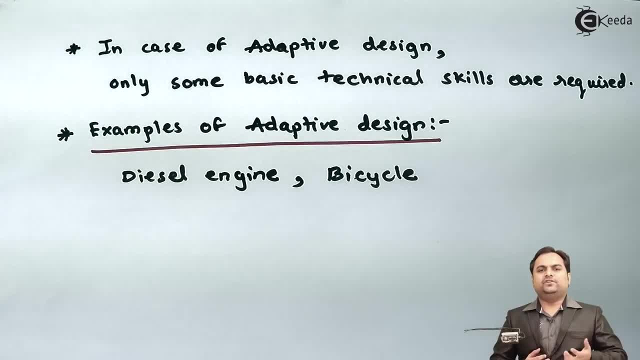 So previously bicycles were existing. then we made small modification in that bicycle by providing gear arrangement, so it became adaptive design. Now we are even having some bicycles which are patented. they operate without the use of the paddle, that is their battery operated. So, as we can see, bicycle was there previously. 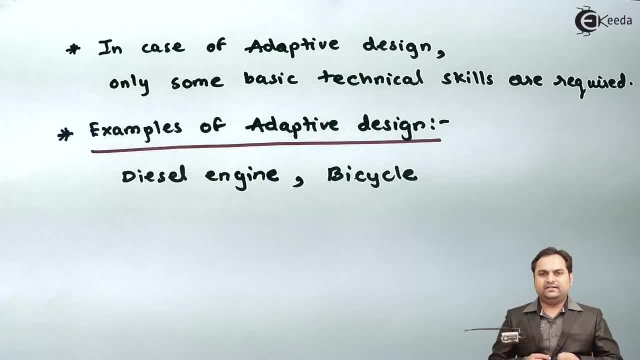 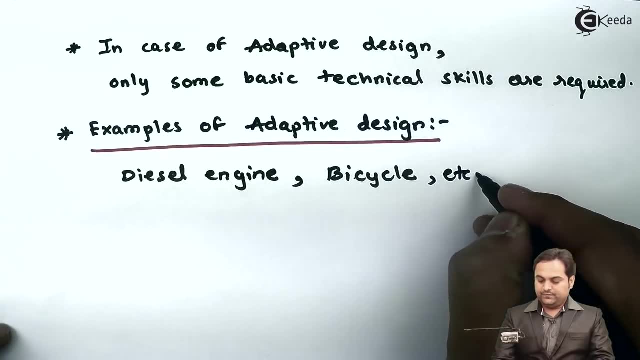 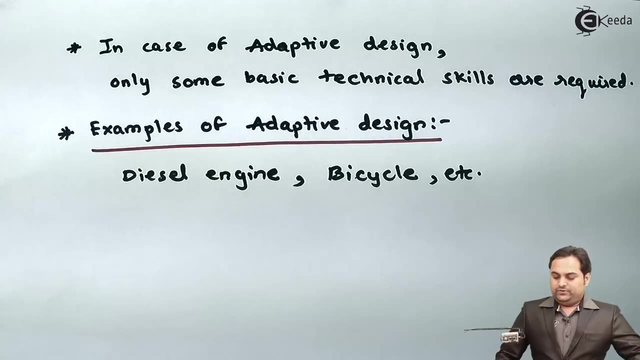 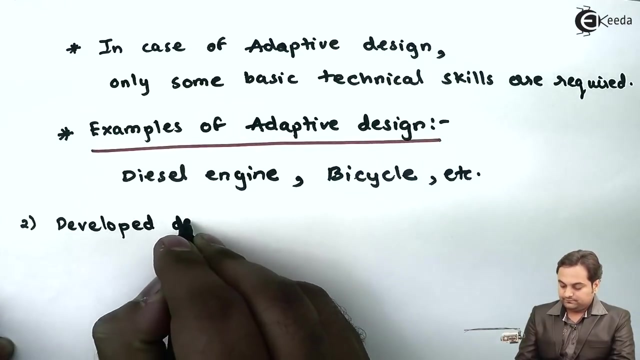 But now We are giving some small, small modifications in that and hence it becomes adaptive design. So these two examples, they are best understood then, etc. we can have number of examples of existing component. then some small changes are made. So this was regarding the adaptive design. next is developed design. 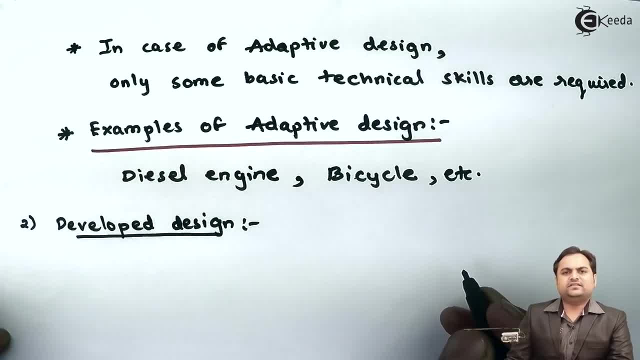 Now when we talk about developed design. Even in this case The existing product is used, but it is used just for the basis, like in adaptive design, the complete product was there and small changes were made. but in developed design the existing product would be used just for an idea and a whole new product would be developed. 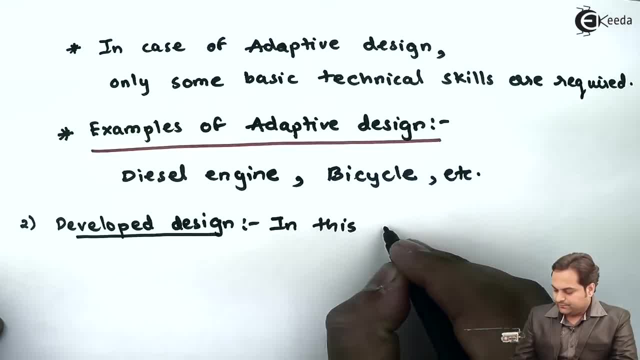 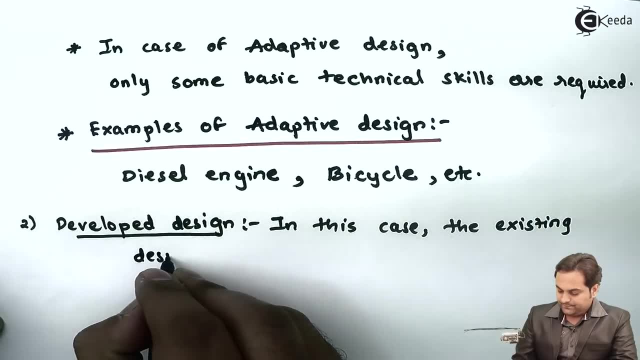 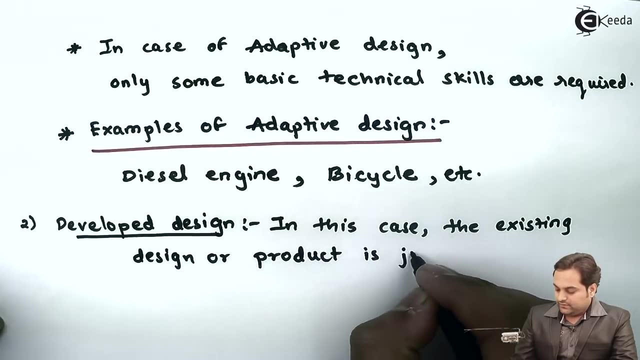 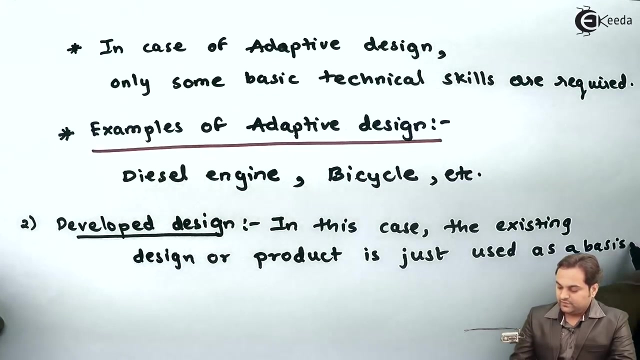 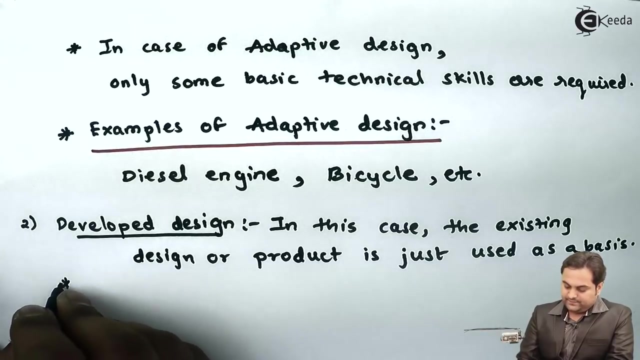 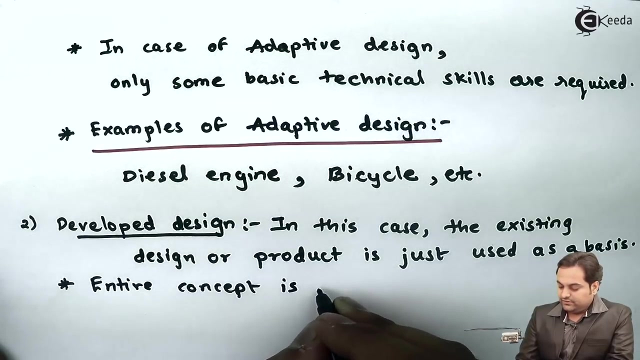 I'll write down, in this case, The existing Design. The existing Design Or product Is Just used As a Basis, Means it would only be used for a reference. Next, Entire Concept Is develop to make a product better. so just by taking the idea of the existing, 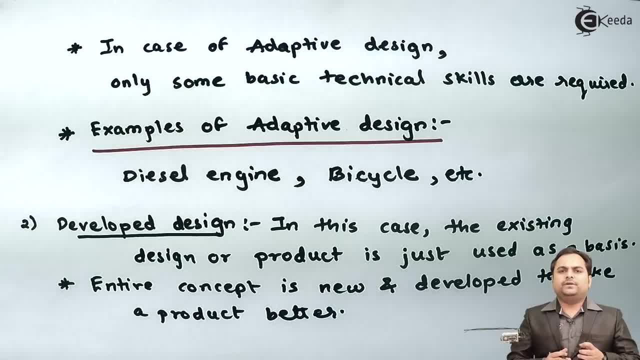 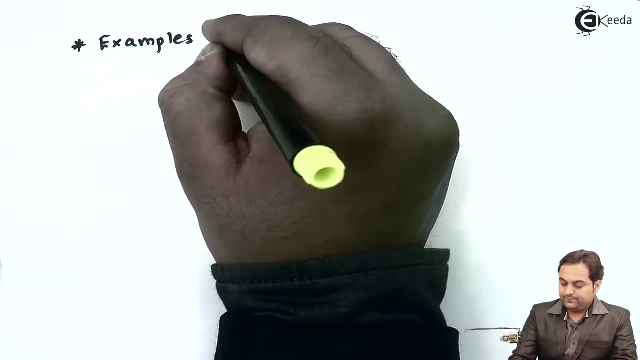 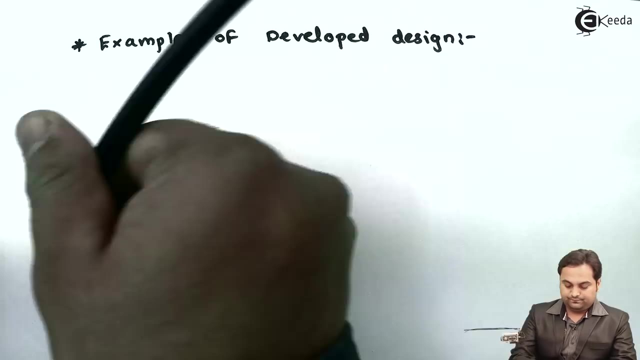 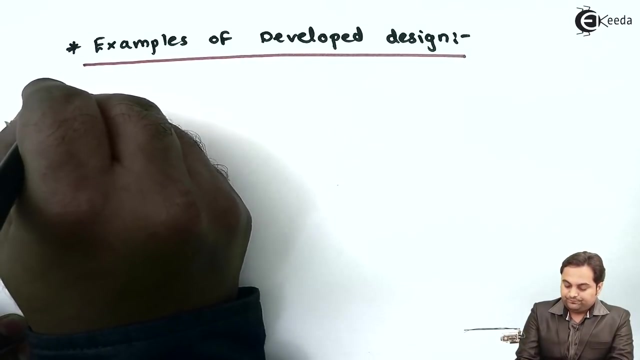 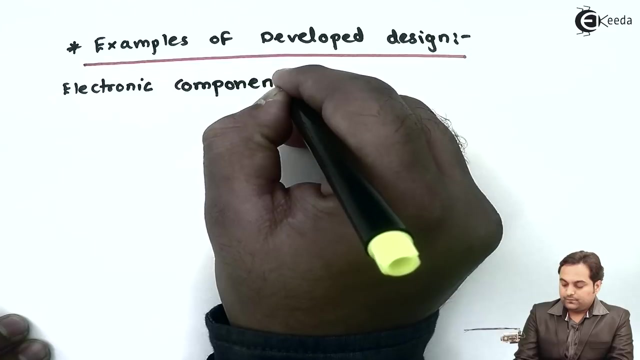 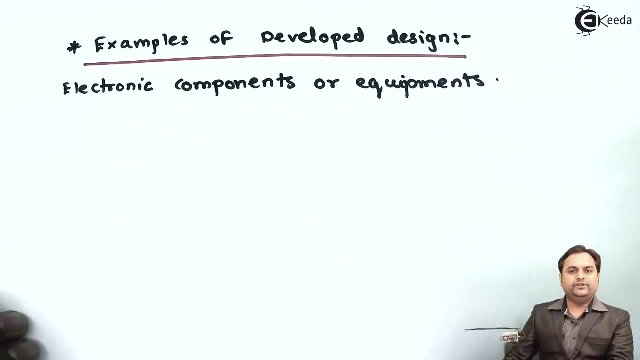 product. we are changing the complete object. that becomes a part of develop design. here I can give the examples. I'll write it on to the next page, the examples of developed design. now, the examples are first of all electronic components or equipments. now see, this is very much understood in today's world that 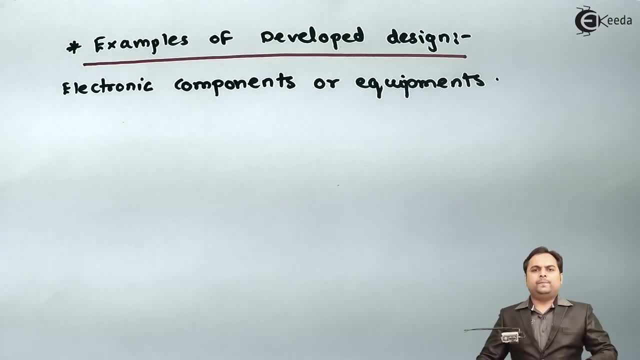 electronic components. if I can take the example of cell phone, we can see number of cell phones which are available with slight modification that is. previously some design was there, it was used as a reference and now we are developing on that, like, as we can see, the Apple phones, like 6 or 6s. they were developed from some earlier version that. 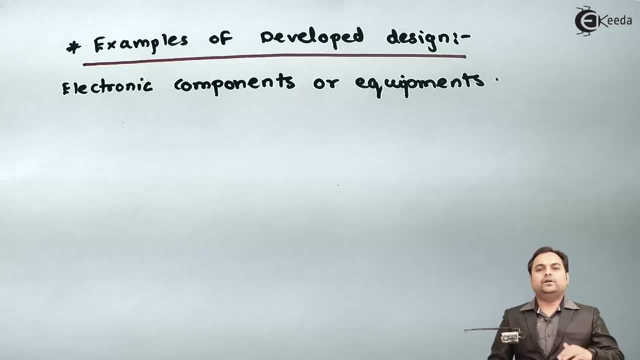 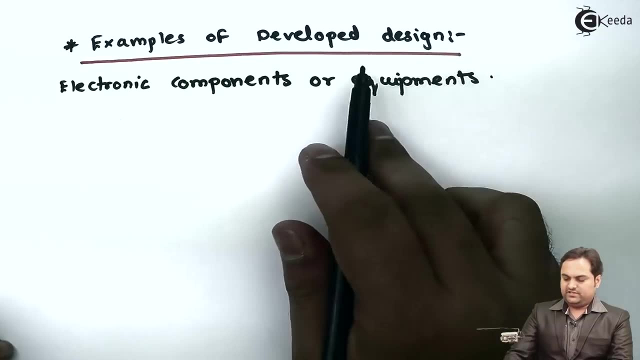 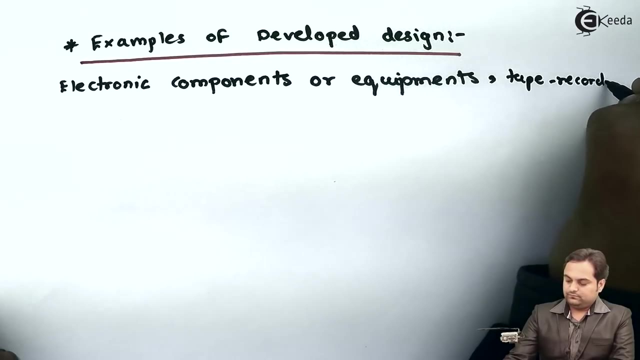 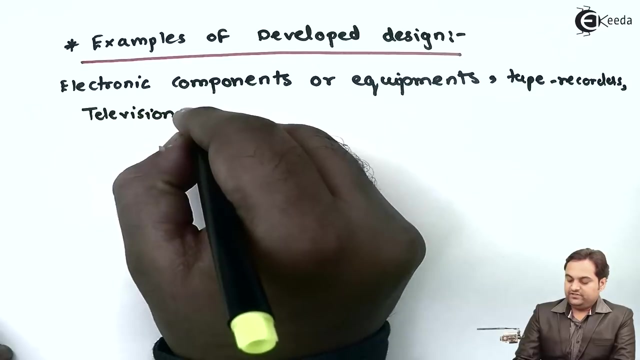 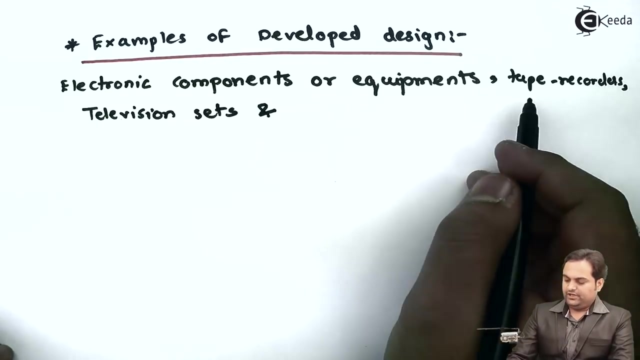 earlier version was acting as a reference and then we developed a complete new design. so that is a part of developed design. so electronic components or equipments, they are the example of develop design. next even tape recorders. then we can say: tape recorders and 곳 calls are all devices and like electronic equipment. 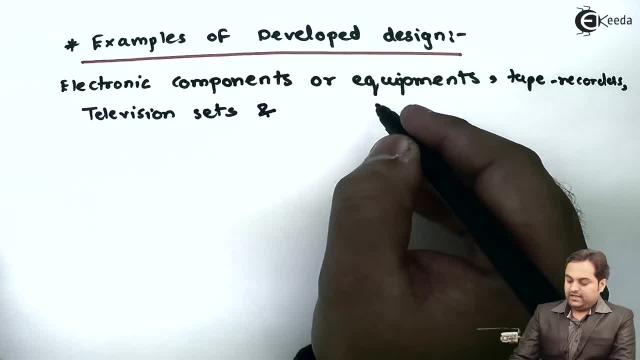 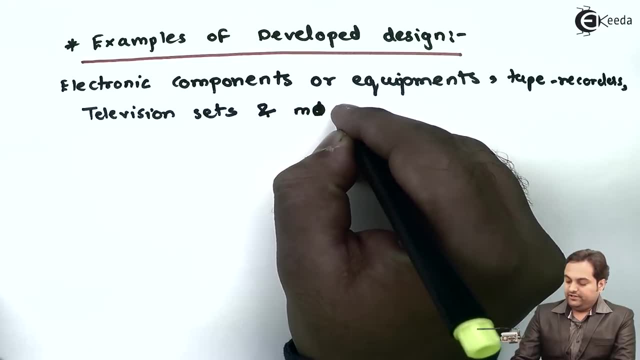 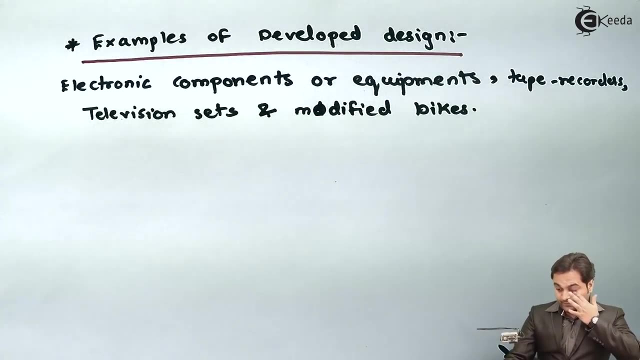 tape record Fall Sh telescope in Kuala Lumpur, Canada. we can also give an example of modified Bytes curtan. like electronic equipment- tape recorders, television sets, and we can even give the erectronic equipment. if you add tape recorders, television sets and we can 해�Rock. 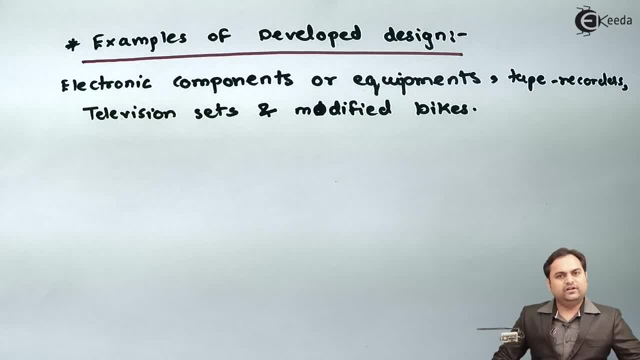 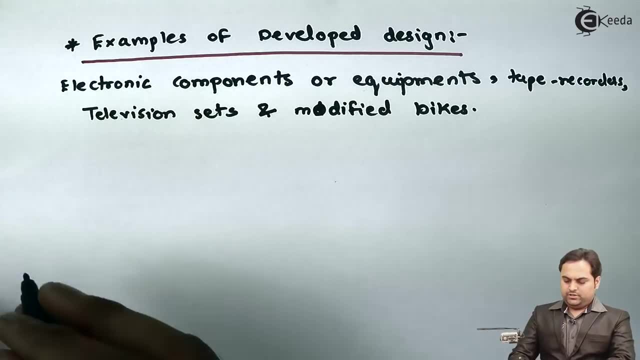 the example off modified bike. so here also, as we have seen these examples, they come apart. like electronic equipment, step recorders, slow down possible processing come under the category of developed design, where we are using the existing model just for the reference and a complete new product is developed. now at last we will see what. 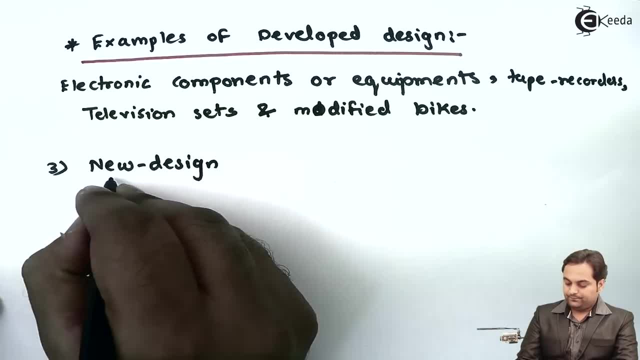 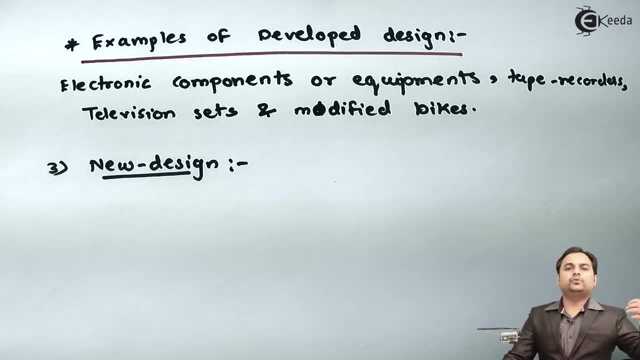 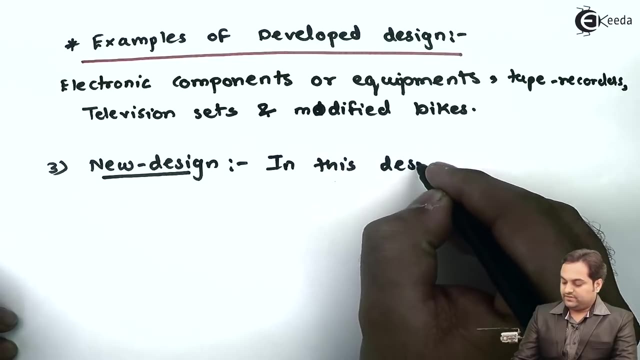 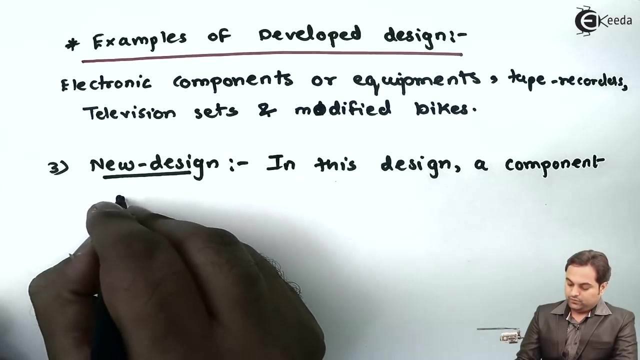 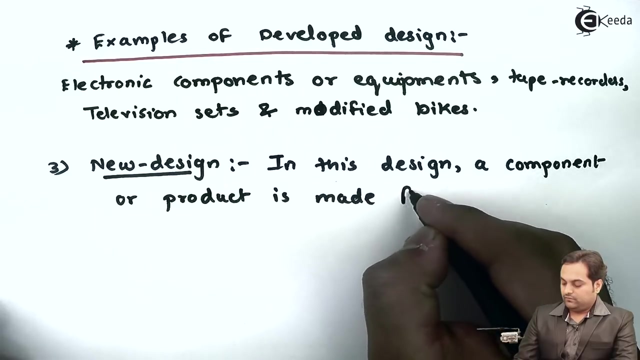 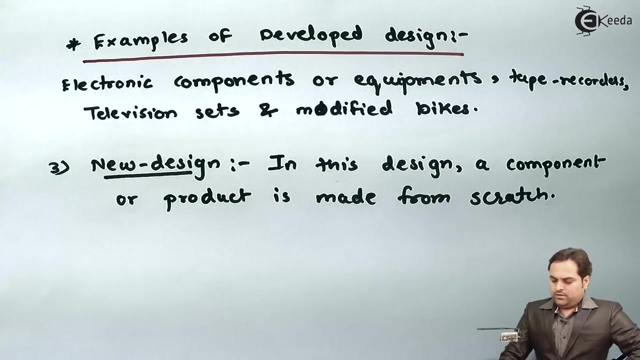 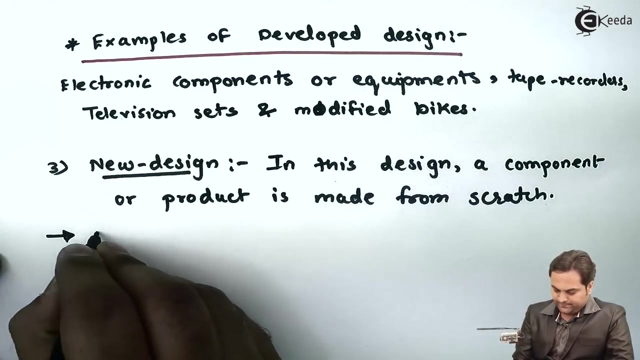 is meant by a new design. in new design, the component is developed as a whole, a new product. here I'll write down: in this design, a component or product is made from scratch, like just starting, and here, as we can see, since we are designing a new component, so the designer, the designer must.